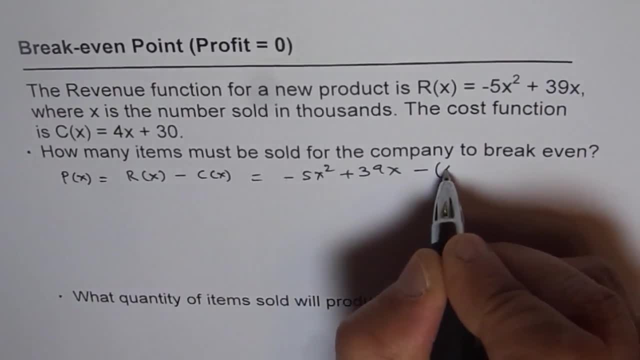 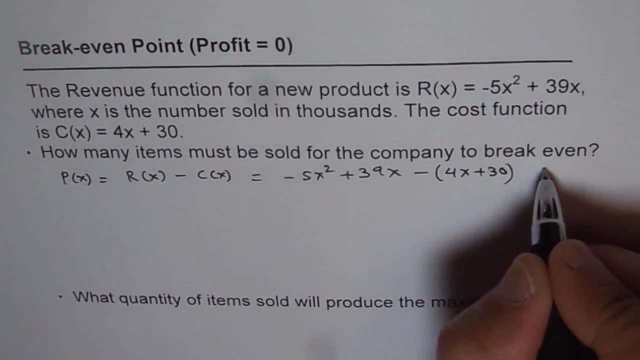 4X plus 30. So let's take away 4X plus 30. Then we get our profit. And now for break-even, all this should be equal to zero, So that becomes our equation. So what we need to do: 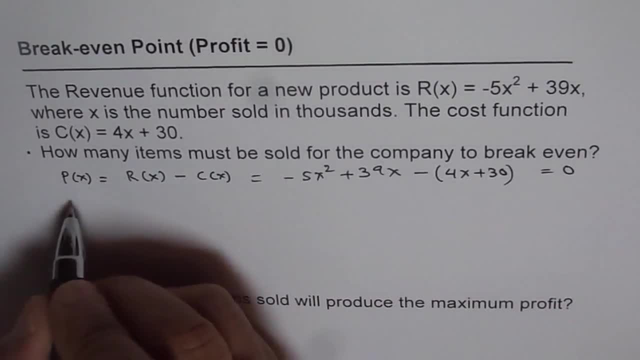 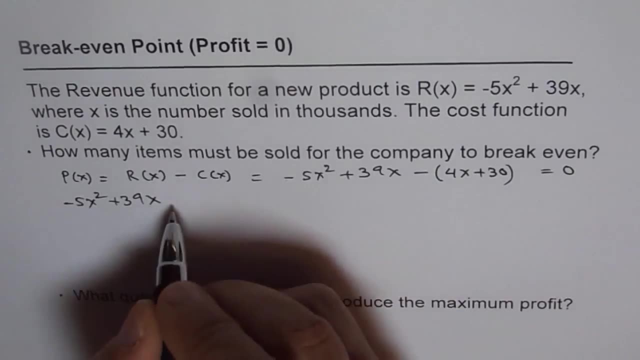 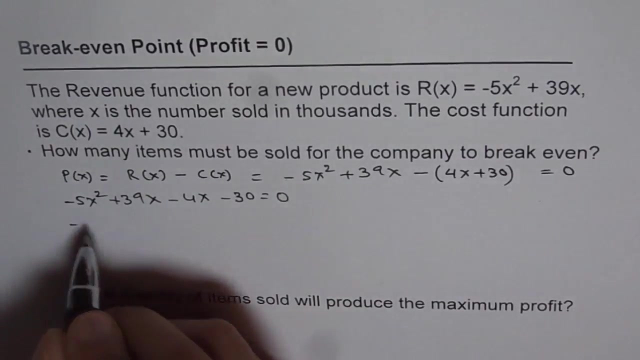 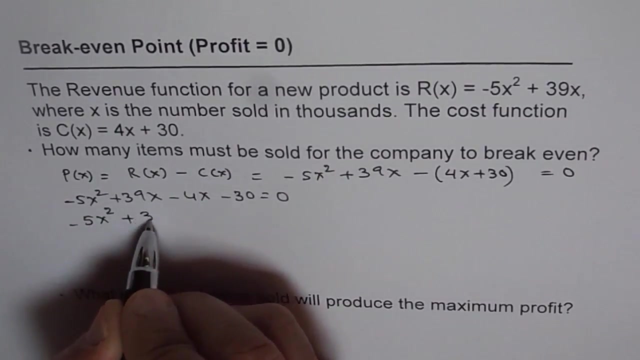 is just simplify this and get the answer. So we have minus 5X squared plus 39X minus 4X minus 30 equals to zero. Now that we can combine these terms, We have 5X squared 39 minus 4 is 35X minus 30 equals to zero. 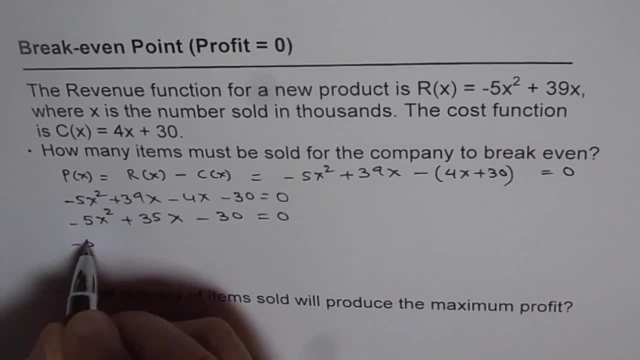 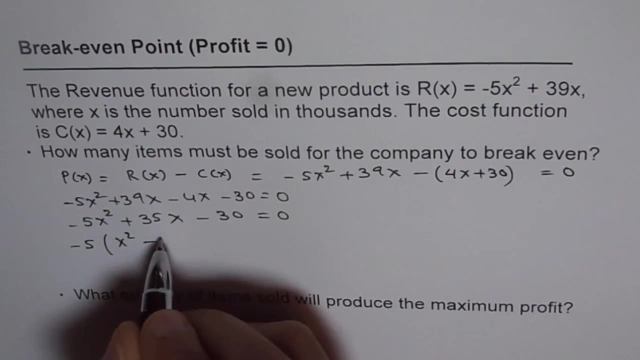 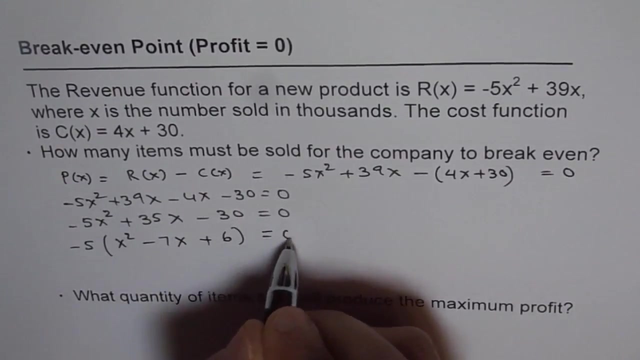 Now we can take 5 common from here, Which is minus 5, and we get X squared. When you take minus, then the signs will change, So this becomes minus 7X And that will be plus 6 equals to zero. Now this can be factored. 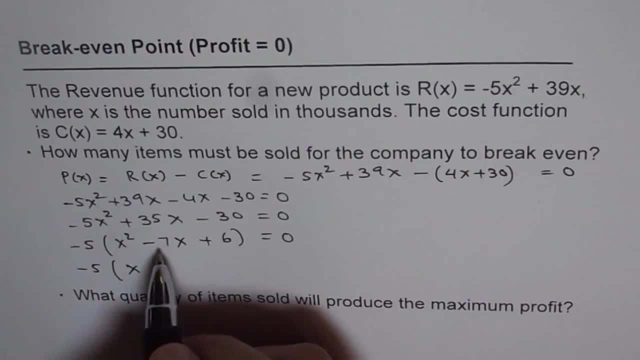 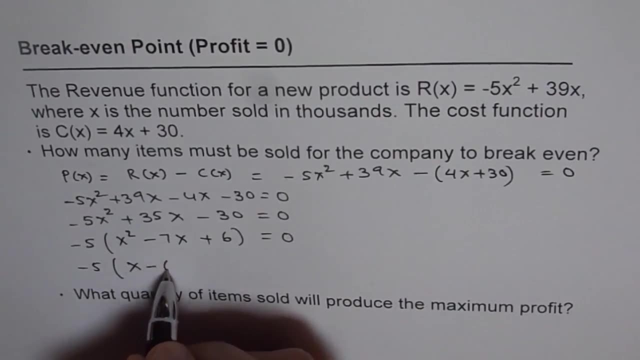 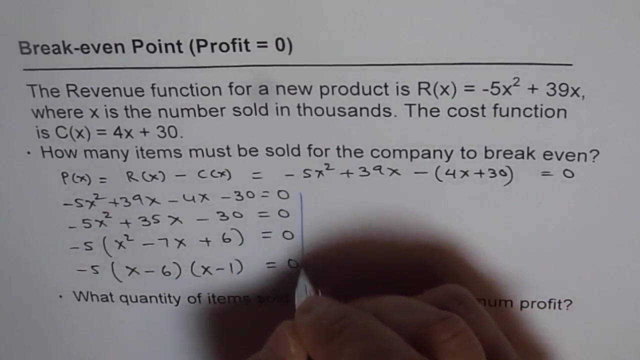 We can write this as X. Now how will you get 7?? You can get it by minus 6 times minus 1, right, So it is minus 6 times minus 1.. So that is how you do it. So this is how you can factor this. Once you have factored, then you can always find the 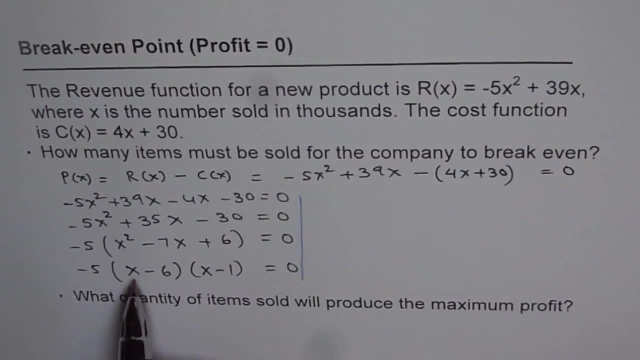 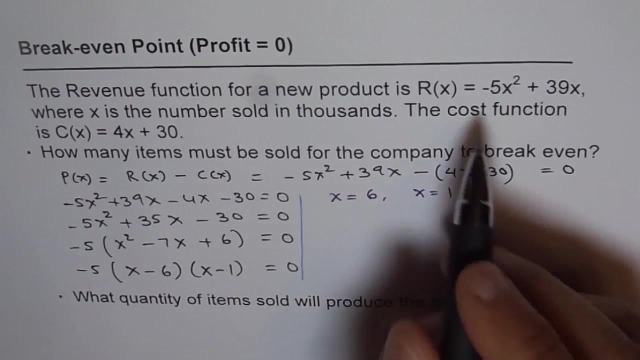 answer. So the answer for us here is: at X equals to 6 and X equals to 1, profit will be zero, right, Profit function will be zero. Now, so that means we get two answers, That is, X equals to 6 and X equals to 1.. Now if you read the question properly, it says where: 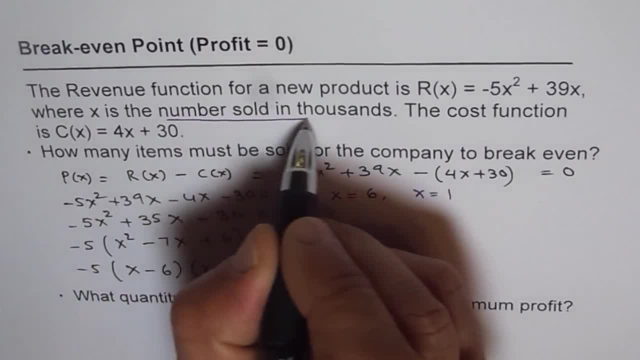 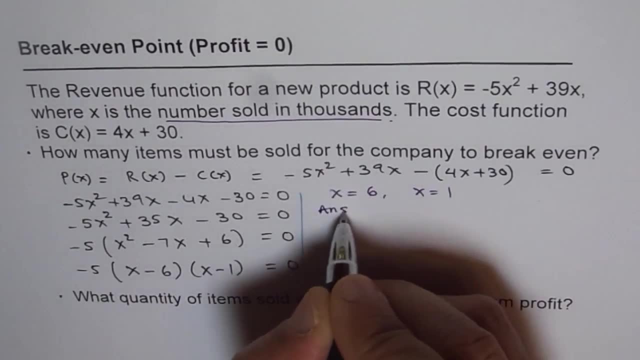 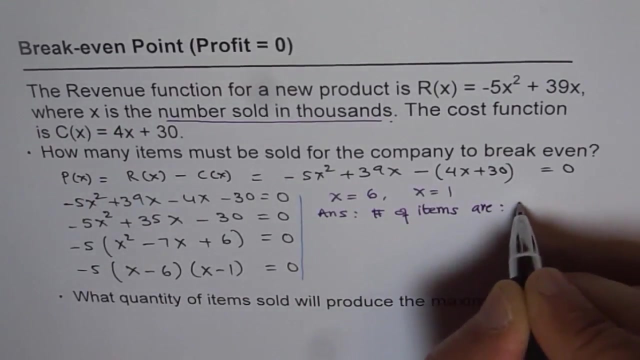 X is numbers sold in thousands, right, Right, Right. So if you write in your answer, you should write that the number of items sold are. so we write down our answer here as number of items are either 6,000 or 1,000, right At. 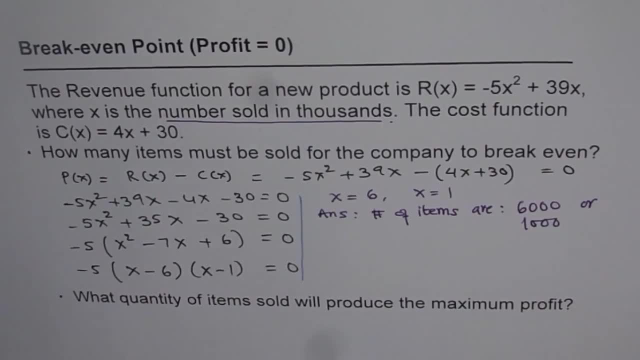 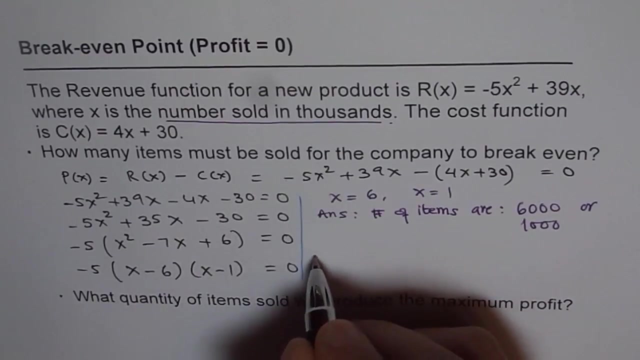 both points, you get a breakeven point right. That is what the answer is Now. part two of the question is what quantity of items sold will produce maximum profit. Now, maximum profit is: this is a profit function, So let's write down the profit function once.